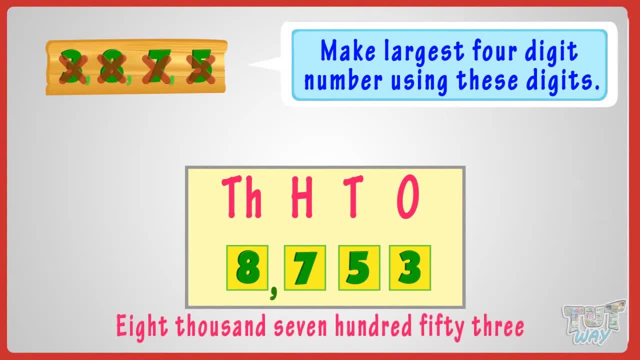 8,753 is the biggest number that we can form using the digits 3,, 8,, 7, and 5.. So, kids, you just need to always arrange the numbers in decreasing order If you want to make the biggest number out of the given numbers. 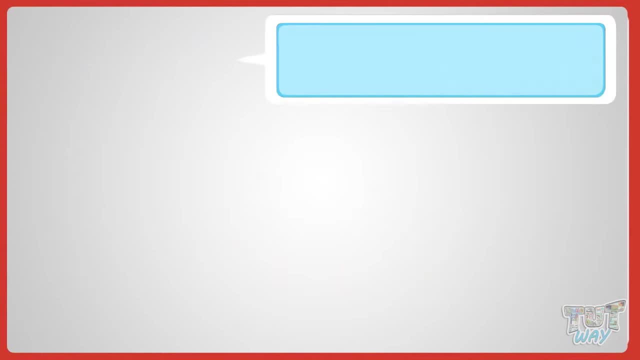 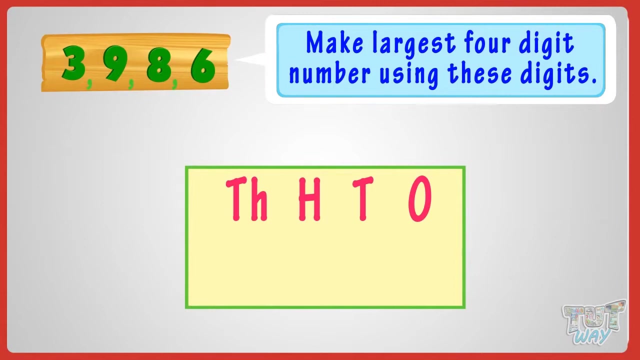 Let's take another example. Here are four numbers. Now We have to make the largest number using these numbers. So arrange the numbers from largest to smallest and your largest number is ready. 9,863 is the number that is made after arranging the numbers in decreasing order. 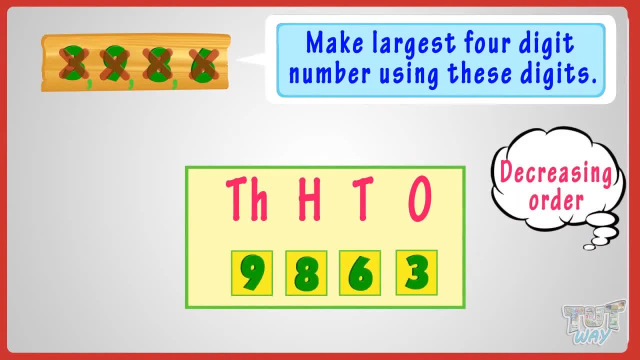 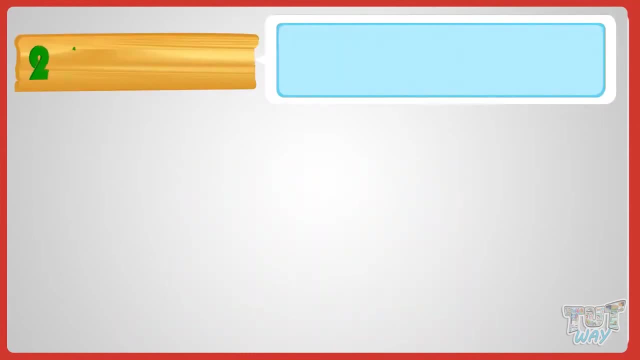 And this is the largest number, And this is the largest number that can be formed: 9,863.. Now let's take another example. Here we have five numbers And we have to make the largest five-digit number using these numbers. 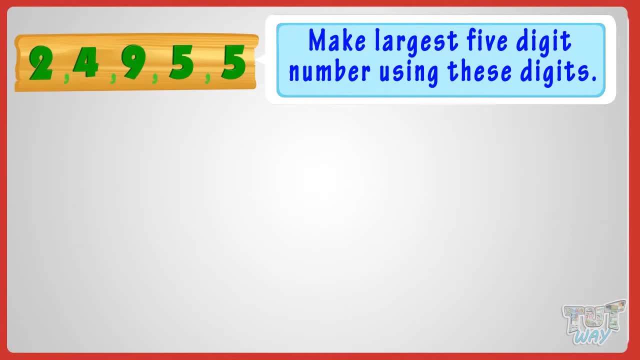 So, kids, you have to arrange the numbers in decreasing order. So we have to arrange the numbers from biggest to smallest To make the bigger number possible using these numbers: 9, 5,, 5,, 4,, 2 is the number that is formed after arranging the numbers in decreasing order. 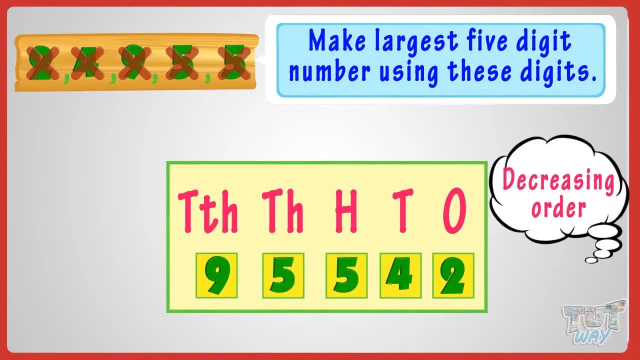 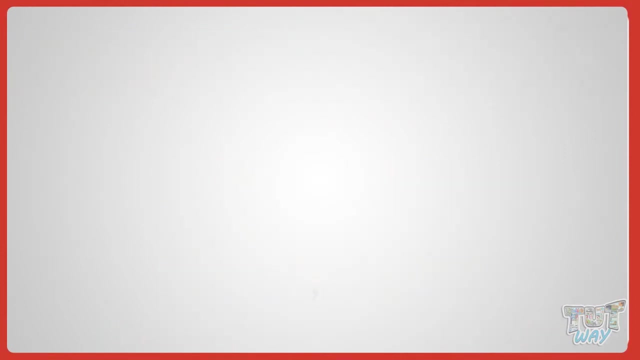 Here 5 comes two times, So we have placed the numbers in decreasing, order them together, So it becomes 95,542, which is the biggest number that can be formed using the given digits. Now let's take another example. Here are four numbers and we have 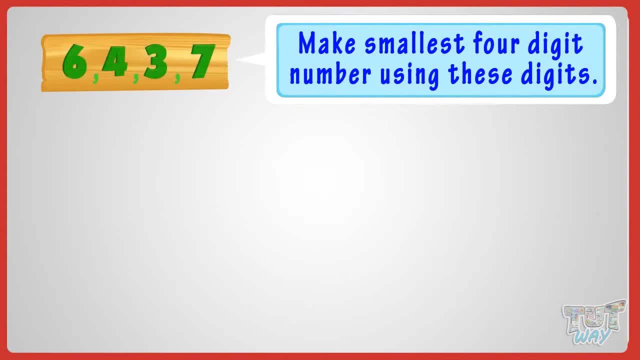 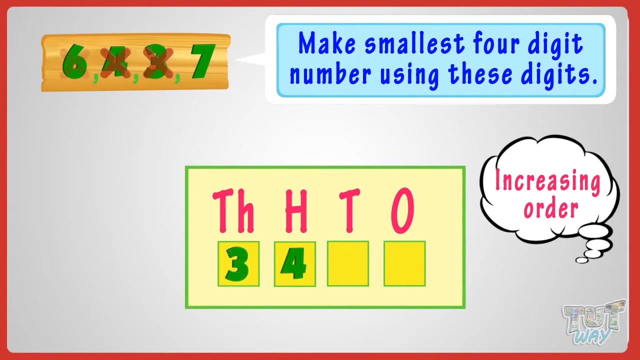 to make the smallest number possible using these numbers. Kids, you have to arrange the numbers from smallest to biggest, That is, in increasing order to make the smallest possible number using the given numbers. So 3, 4,, 6, 7 is the number that we get after arranging. 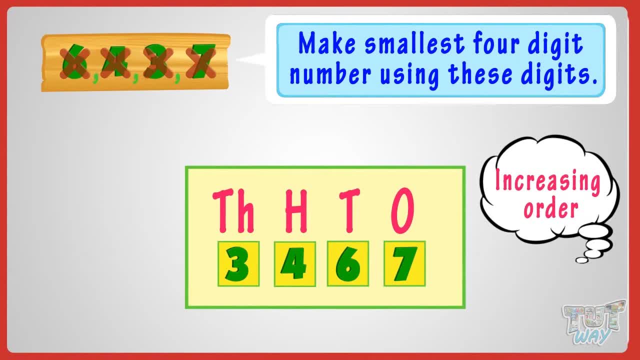 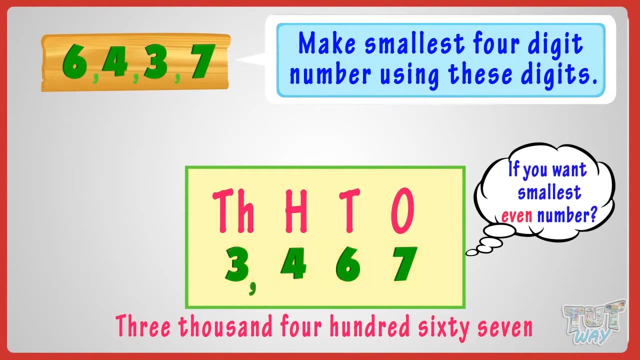 the numbers in increasing order: 3, 467.. This is the smallest number that we can get. Now, if we want the smallest even number, what will you do? Place the biggest even number at the end. The biggest even number we have in the given number is 6.. So place 6 in the end and the rest of the numbers in 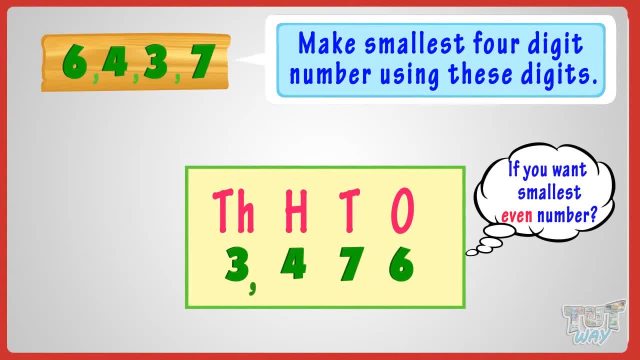 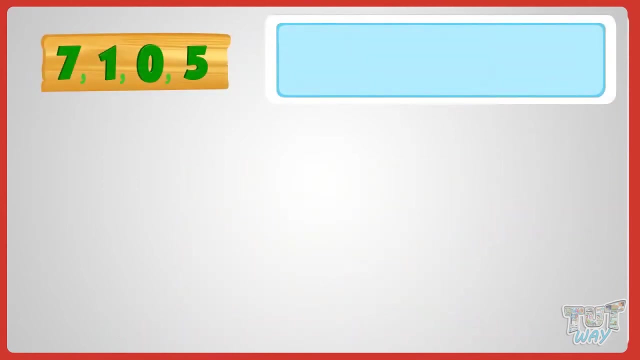 increasing order. So 3, 476 is the smallest even number that we can make using the given numerals. Now let's take another example. Here we have four numerals and we have to make the smallest number possible using the given. 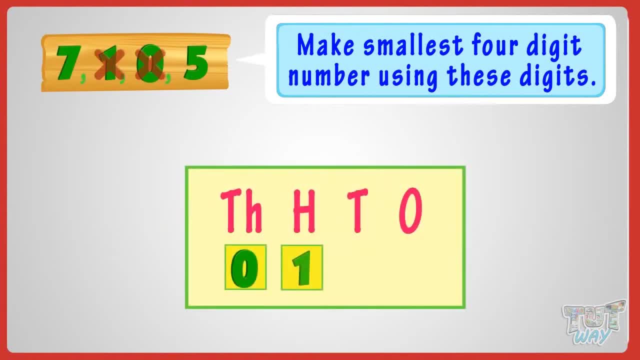 numerals 0,, 1,, 5,, 7 is the number we get on arranging the numerals in increasing order. That is the smallest number possible. Now let's take another example. Here we have four numerals and we have to make the smallest number. 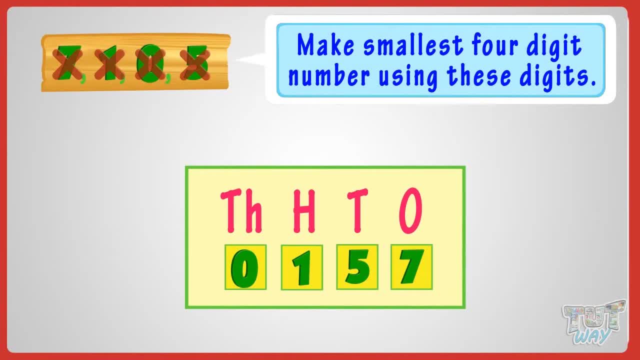 possible To make the smallest even number. make us an even number. We drop 100,000 and the performance seems to be better. But we are asked to make the four digit smallest number. This is gone. We wish to make the 4 digits smallest number. It's not a four digit number as 0,. 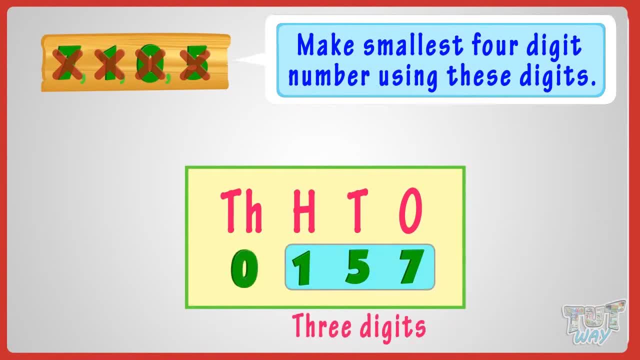 in the beginning makes it a three digit number. So what will we be doing here? Place 0 at the beginning makes it a three digit number: 0 at the next place. that is 10's place. Why? Because there is now 0 right here. So what will we be doing here? Place 0 at.